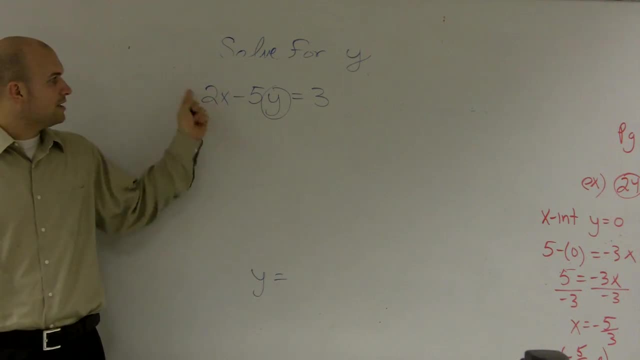 that means I want y all by itself. So we look at what's happening to y. Well, I have a positive 2x, which means I'm adding a 2x, and I have a negative 5 being multiplied by the y. I'm not subtracting. 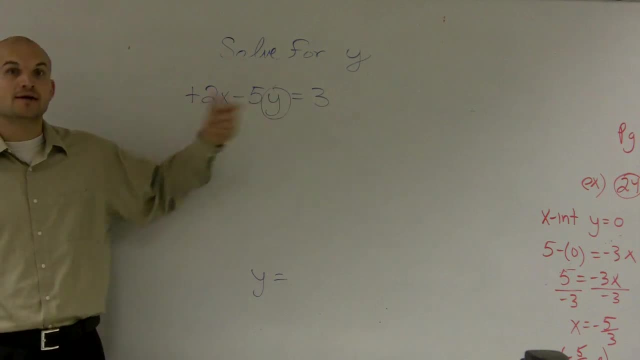 a 5.. That's a negative 5 and it's being multiplied by your y. So the first thing we always do is undo addition and subtraction. So what is being added or subtracted to my variable? Well, I'm adding a equal to y, I'm adding a equal to 5.. I'm adding a equal to y, So I'm adding a equal to y. 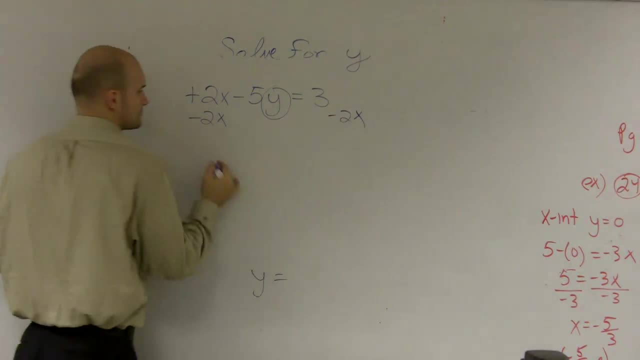 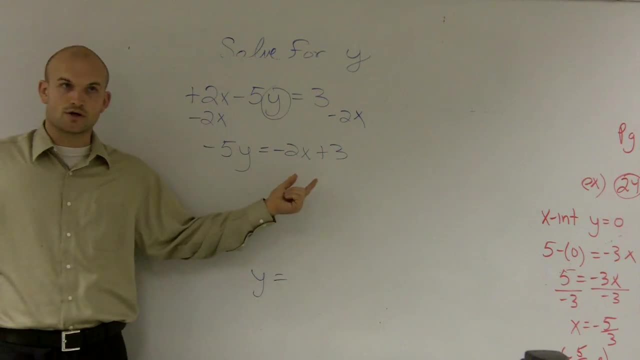 plus 3.. Remember, I told you I always want to write the term with the coefficient or with the variable in it in front of my constant. So that's a positive 3.. That's why it's plus 3.. That's a negative 2x. 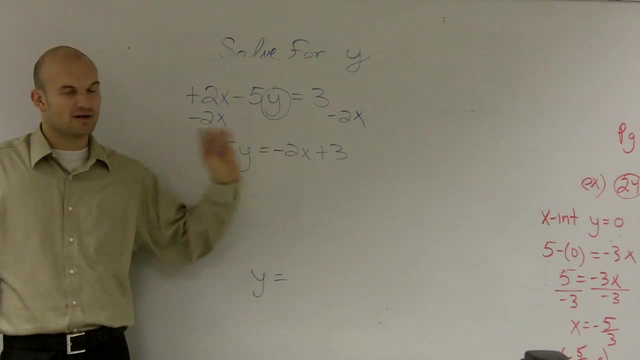 That's why it's negative 2x. And remember you can't combine them. We've already gone over videos on that. You can't combine those two. But now I'm going to divide by negative 5, because negative 5 is multiplied by my y. 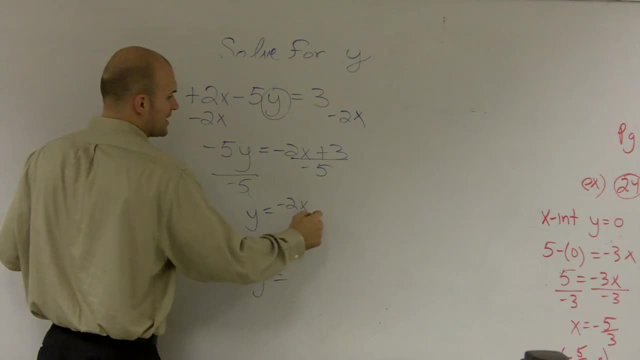 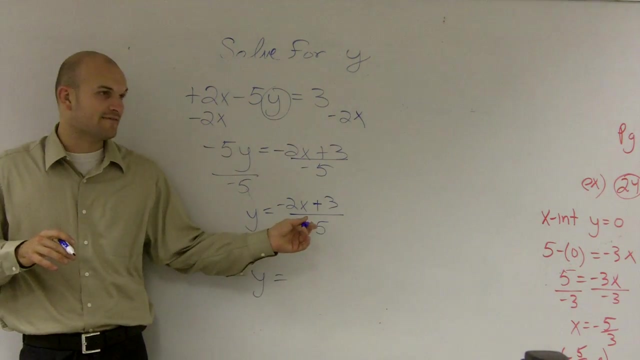 That cancels out to give me 1, so I'm left with: y equals a negative 2x plus 3 divided by 5.. Now, remember, I didn't want this to be my answer. I want you guys to divide that 5 into both of these terms. 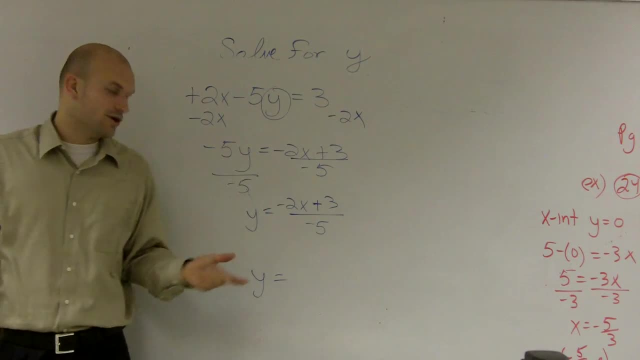 That's a negative 5, right. So now, if you guys notice, negative 5 is not evenly going to negative 2.. So, guess what? We're just going to have a fraction, And that's perfectly fine, because once we learn about slope, you guys will see actually fractions. 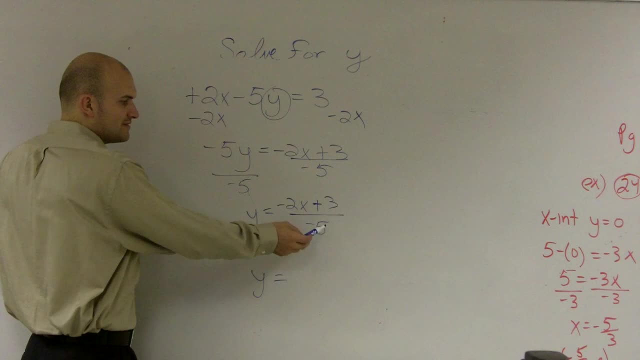 are not that bad. So, Carrie, what you're going to do, and I'm going to say negative 2 divided by negative 5.. The negatives are going to cancel out and I'm left with a positive 2, fifths x. 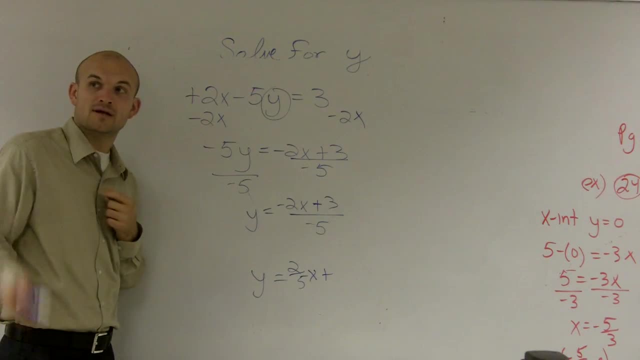 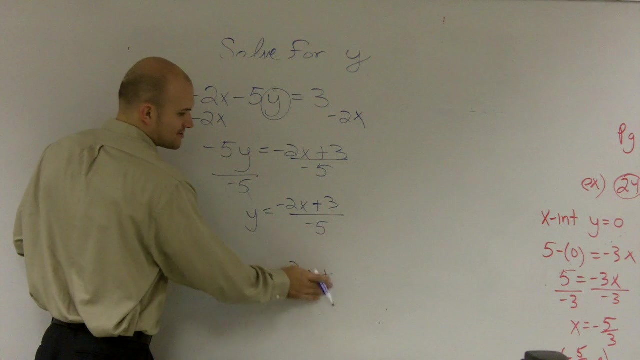 Plus negative 5 does not go into 3 either, so I've got to make up a fraction. But notice, I have a positive 3 divided by negative 5.. So that's going to be a negative 3 fifths, Or I can just write minus 3 fifths. 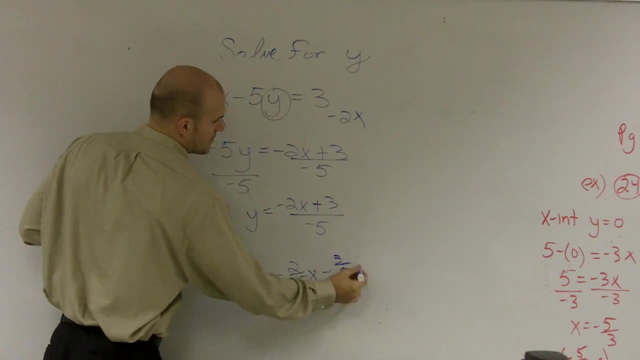 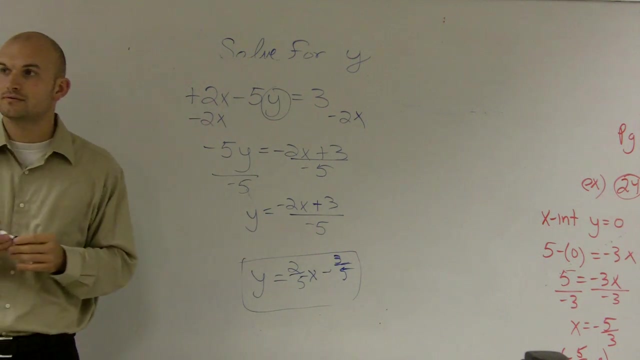 So that would be how I want you to write your finalized answer. So that's how you solve for y when you have a problem with an x and a y. 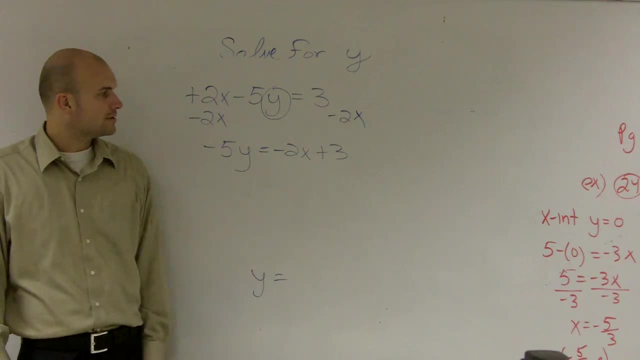 or with the variable in it in front of my constant. So that's a positive 3.. That's why it's plus 3. That's a negative 2x. That's why it's negative 2x. And remember you can't combine them. 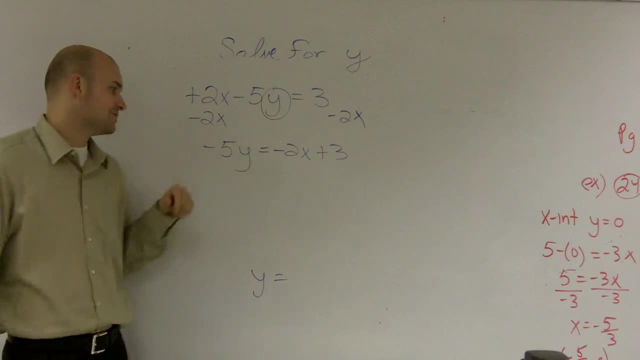 We've already gone over videos on that. You can't combine those two. But now I'm going to divide by negative 5, because negative 5 is multiplied by my y, That cancels out to give me 1, so I'm 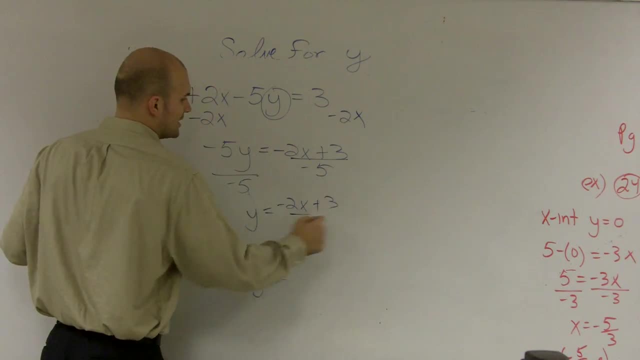 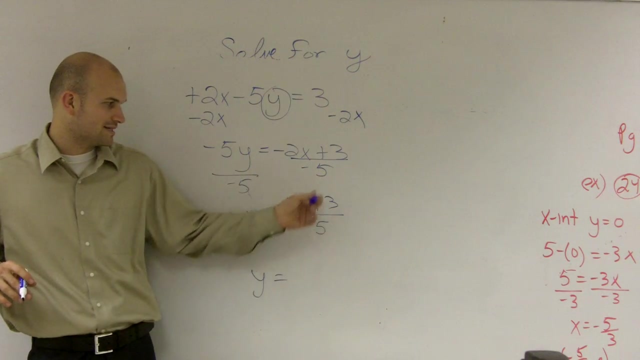 left with y equals a negative 2x plus 3 divided by 5.. Now, remember, I didn't want this to be my answer. I want you guys to divide that 5 into both of these terms. That's a negative 5, right. 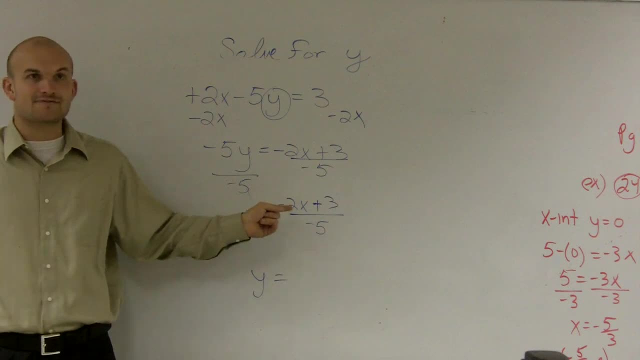 So now if you guys notice, negative 5 is not evenly going to negative 2.. So guess what? We're just going to have a fraction, And that's perfectly fine, because once we learn about slope you guys will see actually fractions. 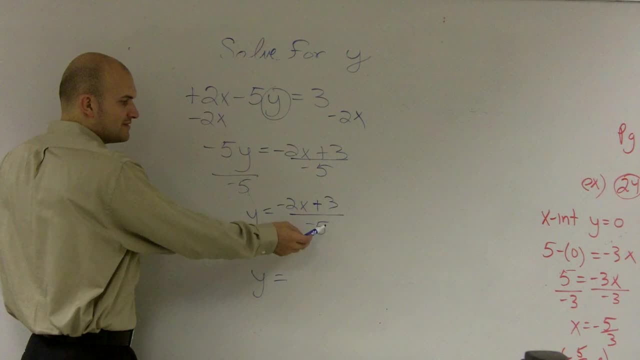 are not that bad. So, Carrie, what you're going to do, and I'm going to say negative 2 divided by negative 5.. The negatives are going to cancel out and I'm left with a positive 2, fifths x. 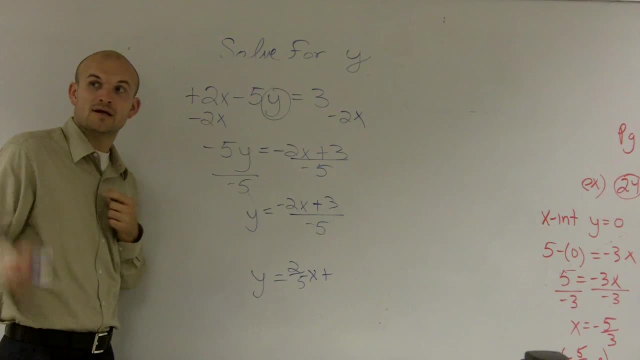 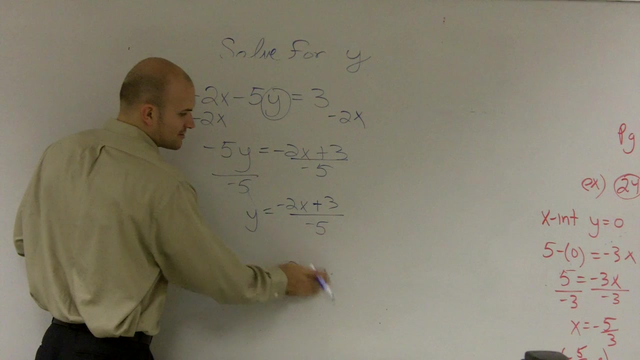 Plus negative 5 does not go into 3 either, so I've got to make up a fraction. But notice, I have a positive 3 divided by negative 5.. So that's going to be a negative 3. fifths: 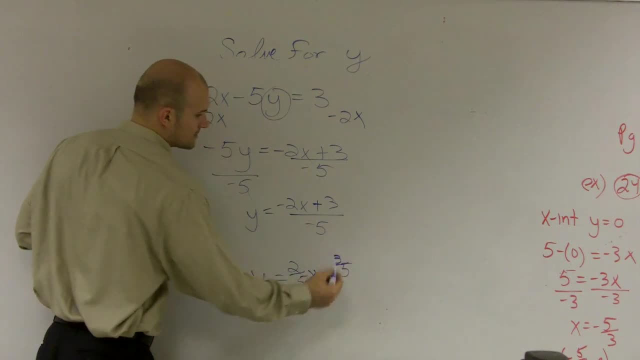 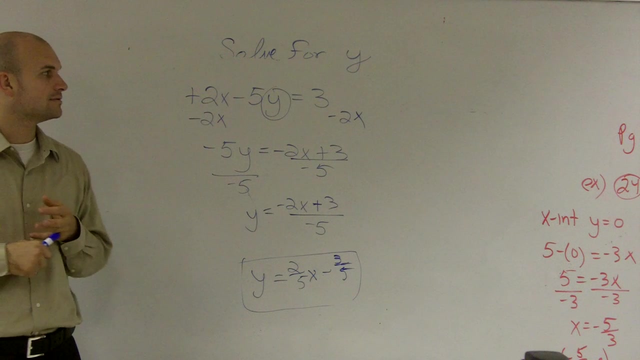 Or I can just write minus 3 fifths, So that would be how I want you to write your finalized answer. So that's how you solve for y when you have a problem with an x and a y. There we go- Wow time.